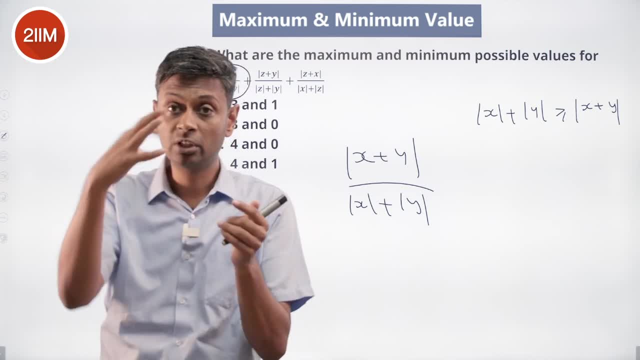 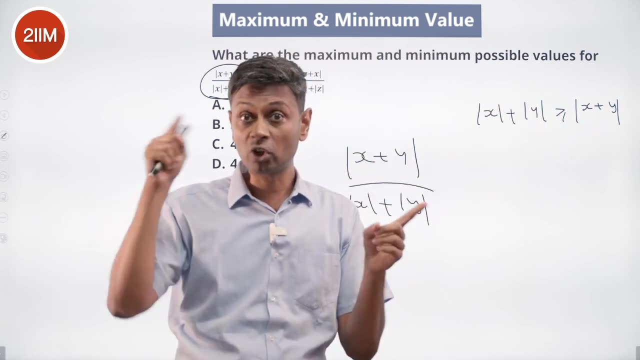 adding the two numbers. We are adding two numbers. If one number is positive, other is negative, the magnitude will shrink. Mod 5 plus mod 3 is mod of 5 plus 3.. Mod 5 plus mod of minus 3. 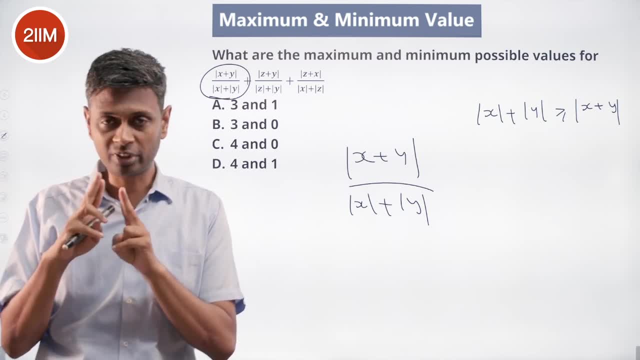 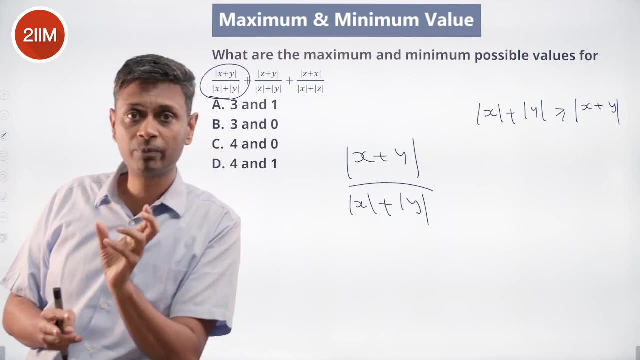 will be greater than modulus of 5 minus 3.. x and y have opposite signs, Then their magnitude will kind of cancel each other, partly at least, And then modulus of x plus y will shrink, whereas mod x plus mod y is sum of the two magnitudes. When will it be equal? 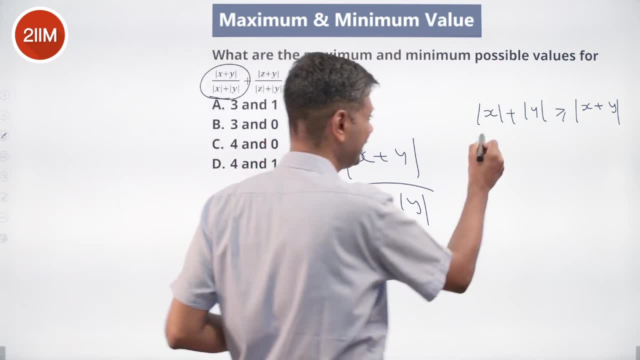 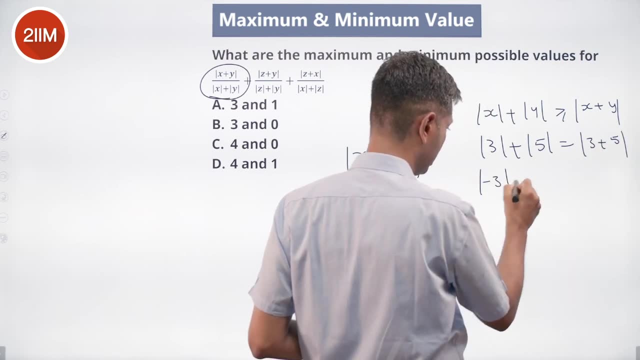 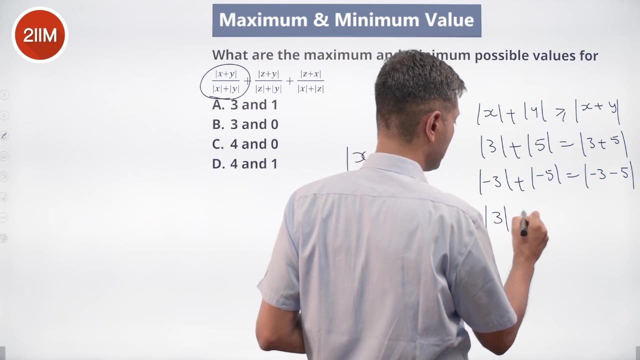 It will be equal when they have the same sign. So lovely idea. Mod 3 plus mod 5 is equal to modulus of 3 plus 5.. Mod minus 3 plus mod minus 5 is equal to modulus of minus 3 minus 5.. Mod 3 plus mod of 5.. 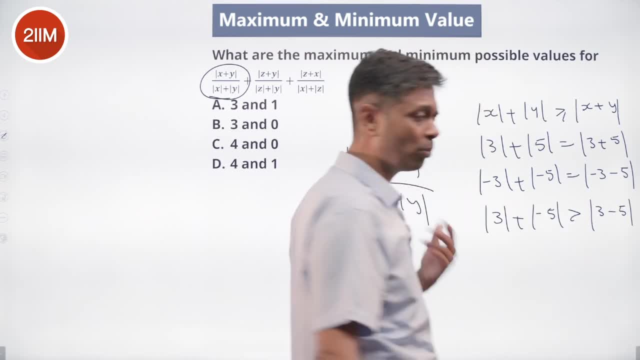 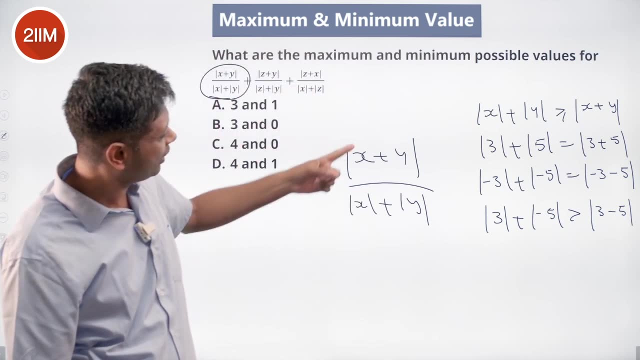 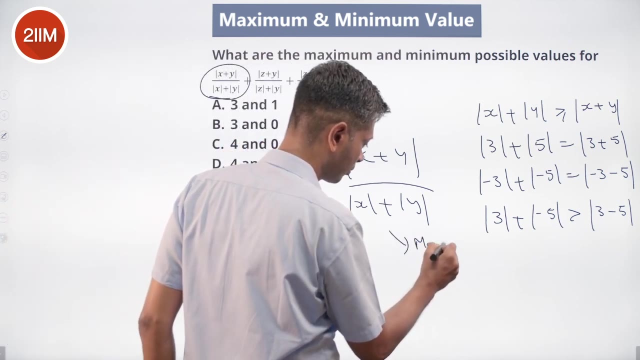 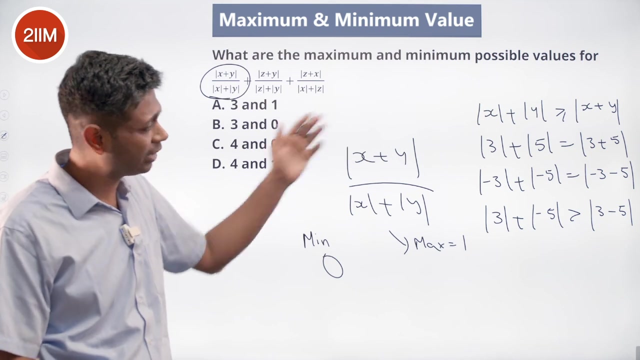 minus pi greater than modulus of 3 minus pi. We have opposite signs. It crashes out, It becomes smaller. These two will be greater. So mod of x plus y by mod x plus mod y will be 1.. Maximum equal to 1.. What is the minimum? It will be 0.. Because modulus of x plus y 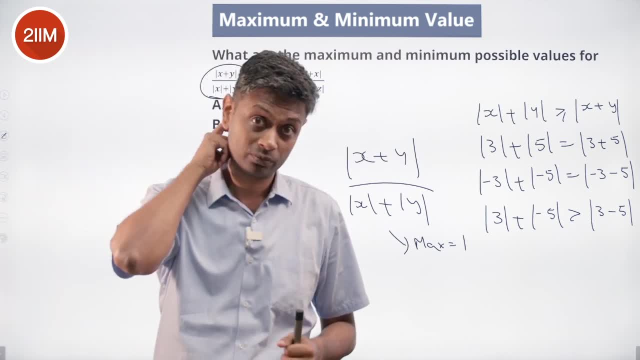 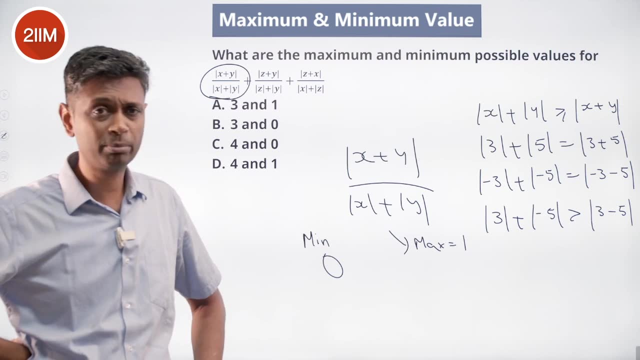 can go to 0.. When x is equal to minus 1, it can go to 0.. Brilliant Modulus of x plus y can go to 0.. Modulus of 3 plus minus 3 is 0.. So each of these expressions goes from. 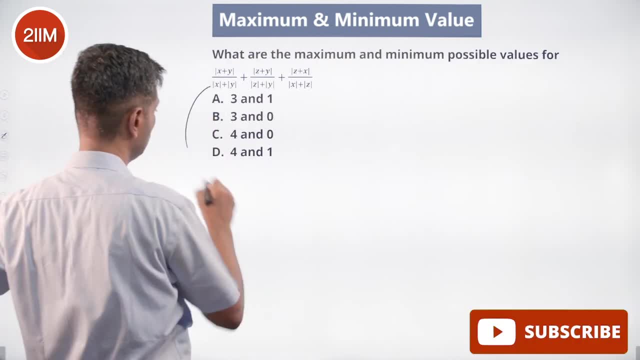 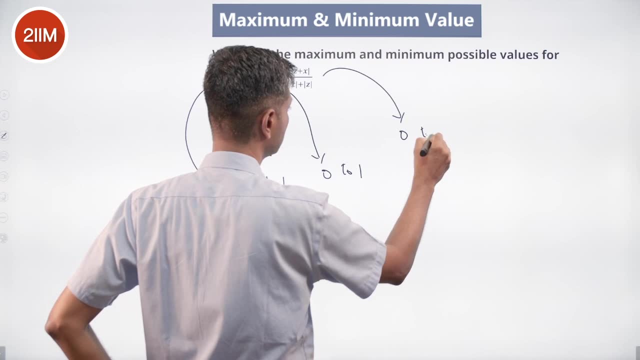 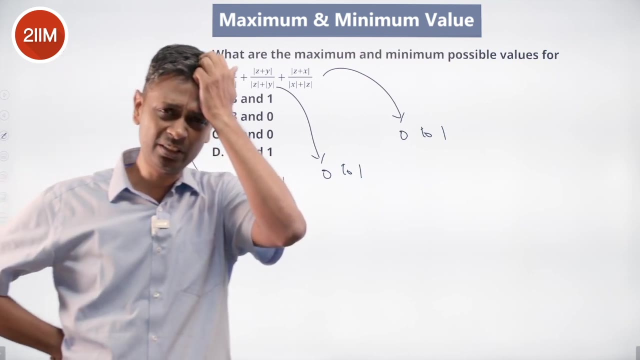 0 to 1.. This goes from 0 to 1.. This goes from 0 to 1.. This goes from 0 to 1.. Nice, Very interesting. So the overall term total should go from 0 to 3.. Maximum is 3.. Minimum is 0.. Now, when will the maximum happen? 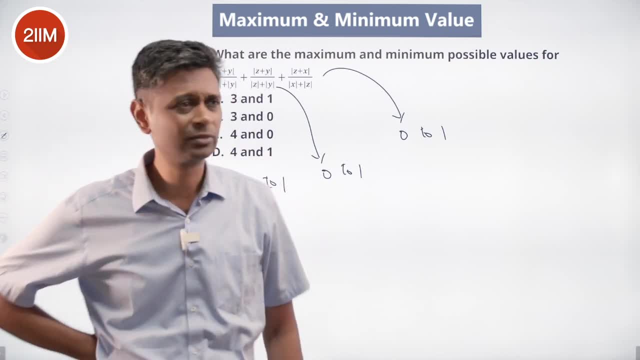 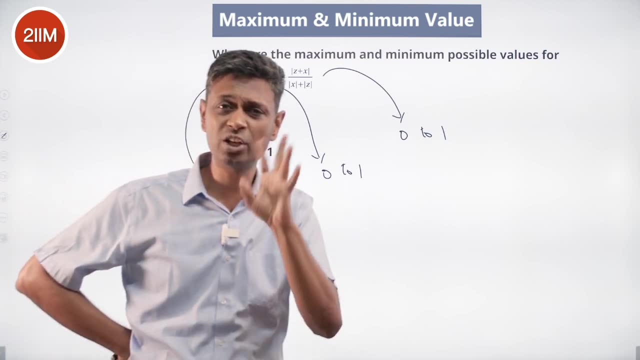 Suppose I put x is 2, y is 3, z is 4.. 2 plus 3 by 2 plus 3.. 3 plus 4 by 3 plus 4.. 2 plus 4 by 2 plus 4.. Brilliant 3 is possible. Can I get 0, 0, 0?? Is that even possible? That's. 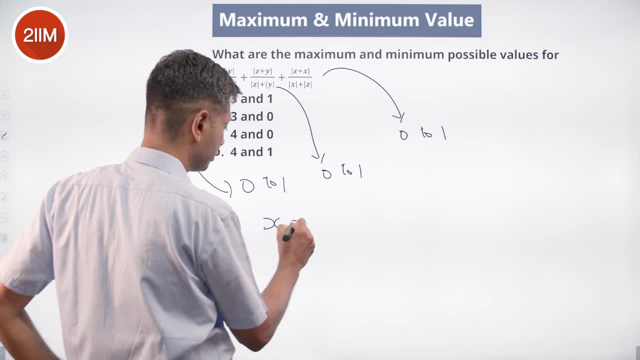 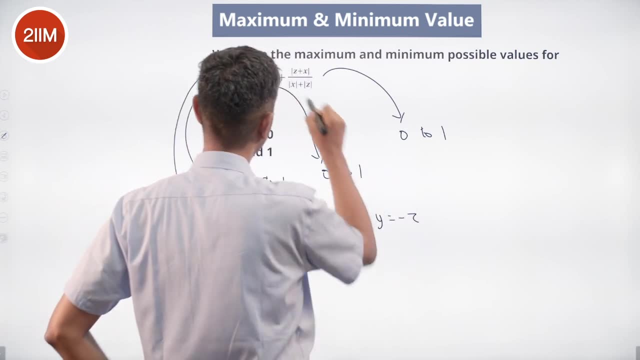 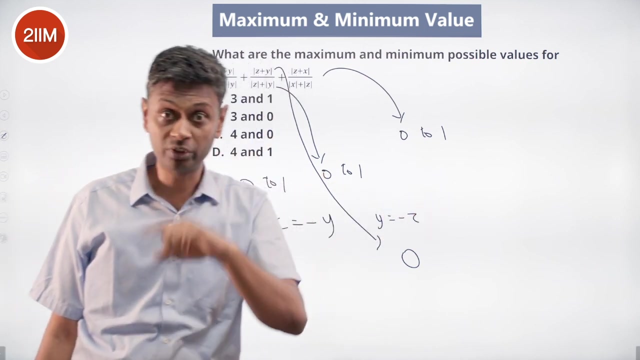 where it becomes funny, Because if I put x equal to minus y, this will go to 0.. Let me put y equal to minus z, This will go to 0.. y is minus x and minus z. That means x should be equal to z. Here again, I cannot say z equal to x, z equal to minus x, That's. 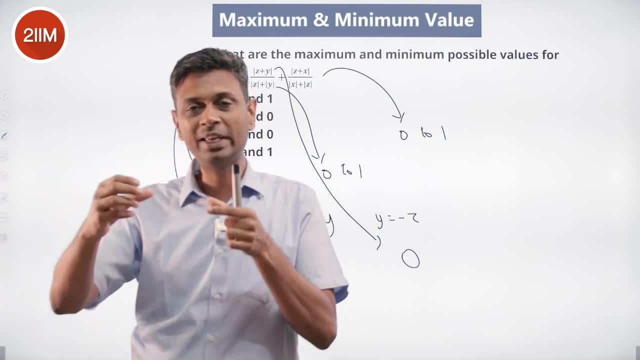 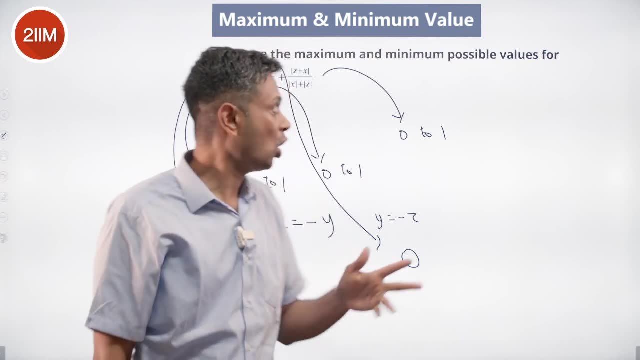 not possible. x, y and z, x and y can have opposite signs. y and z can have opposite signs. Again, x and z also cannot have opposite signs. Of the 3 numbers, all 3 can be positive. all 3 can be negative. 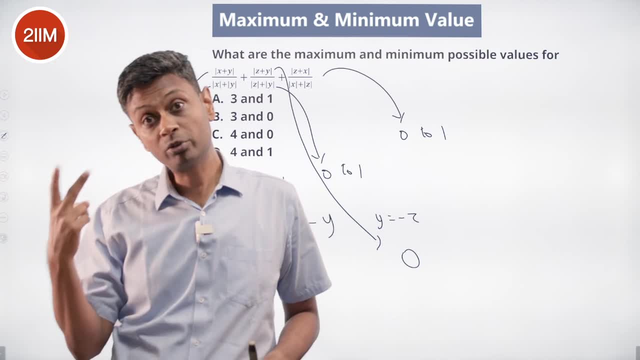 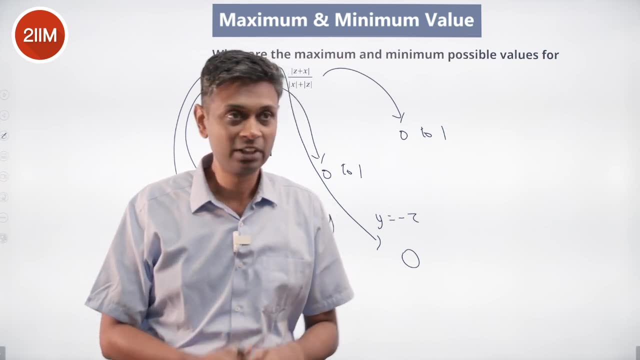 In which case it will add up to 3.. Nice, 2 can be positive, 1 can be negative. 2 negative, 1 positive: The sum of 2 numbers at least that have the same sign, In which case it 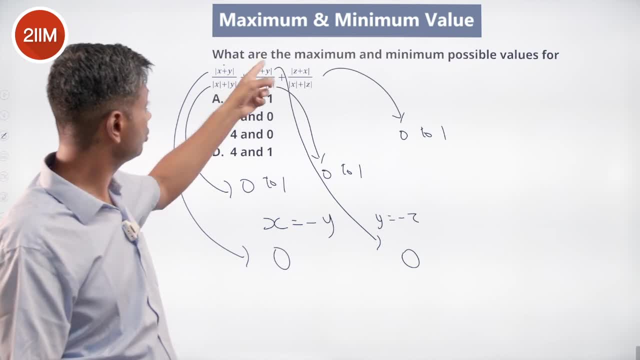 cannot go to 0. You cannot have a scenario where this goes to 0, this goes to 0 and this goes to 0. That's not possible. I can make 2 of them go to 0. In which case, the third. 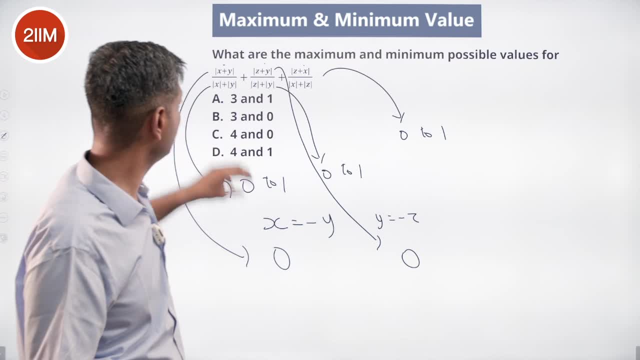 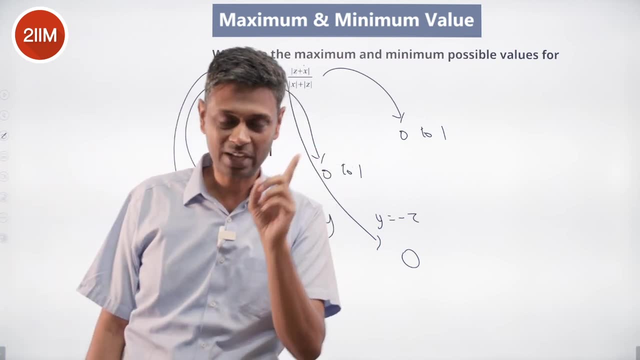 one will end up being 1.. So I can have a mechanism where these 2 go to 0, in which case this will be 1.. These 2 go to 0, in which case this will be 1.. 1 of the 3 has to be 1.. I cannot have all 3 numbers, every pair having different sign. 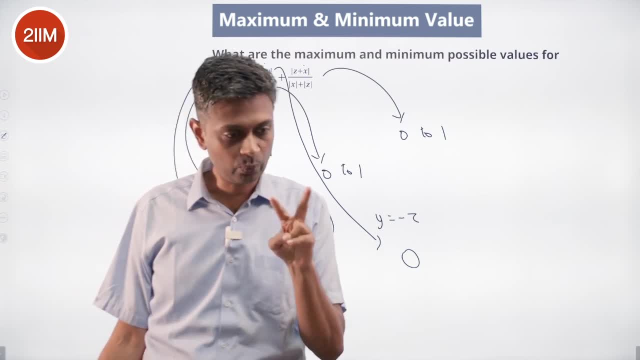 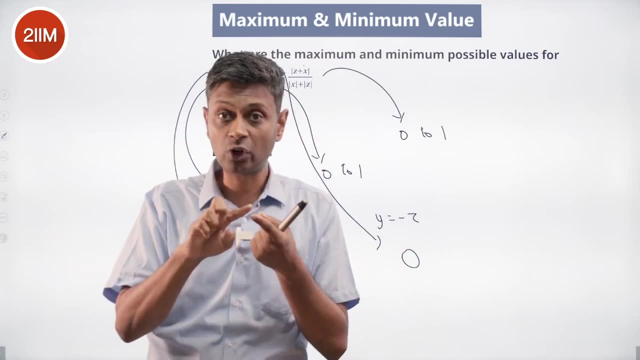 I cannot have plus and minus, plus and minus, plus and minus. That's not possible. If x and y have opposite signs and y and z have opposite signs, that means x and z should have the same sign. I cannot have x and y having opposite signs, y and z having opposite. 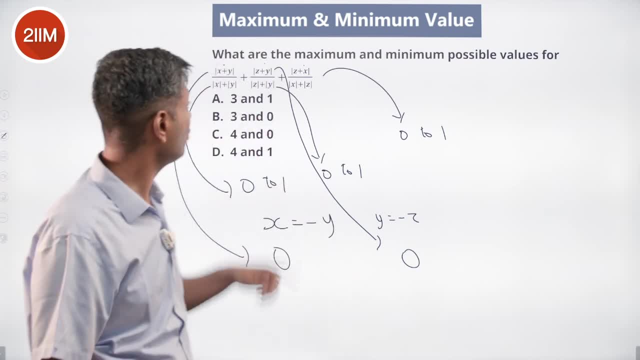 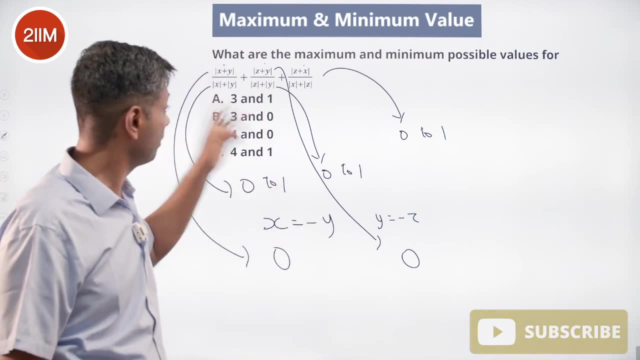 signs z and x have opposite signs. That's not possible. So of these 3 terms, at least 1 of them is equal to 1.. So the minimum is 1, maximum is 3.. When will it be 3?? I put x equal to 2, y equal to 3,. 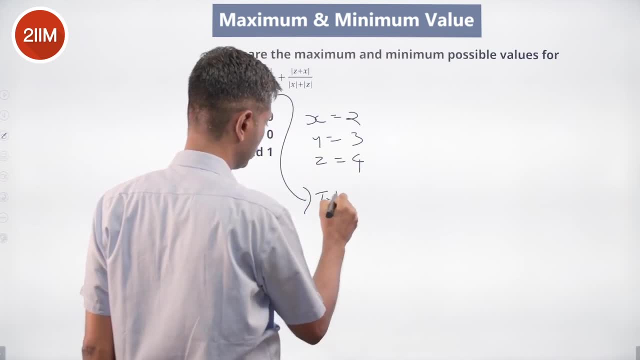 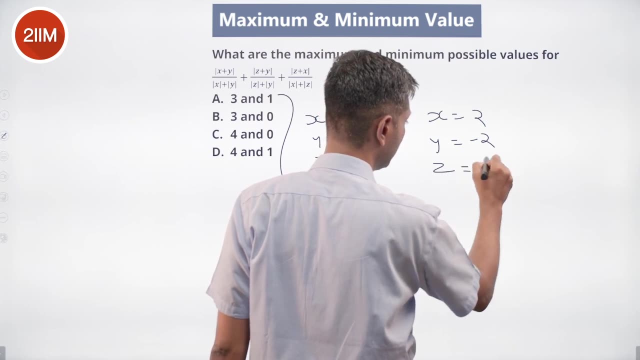 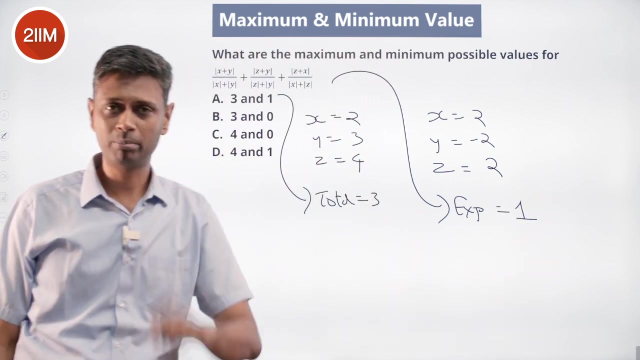 z equal to 4.. This expression, total, would be 3.. I put x equal to 2,, y equal to minus 2, z equal to 2.. This expression will be equal to 1.. Minimum is 1, maximum is 3.. Below, 1 is not.